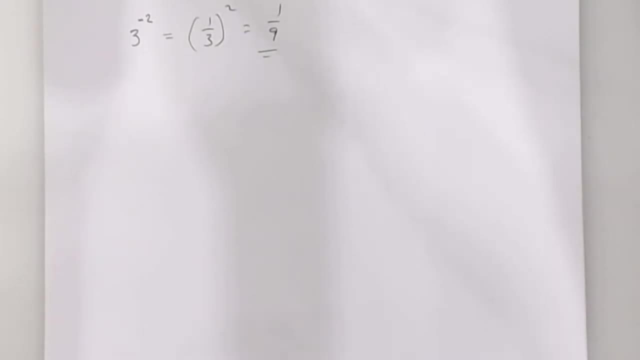 Okay, so we talked about negative exponents yesterday. We had like two problems like that. Now it's going to take us with the question I'm about to ask you about exponential functions in a little while, So when we're let's look at this one. what if you had three-fourths to the negative third power? 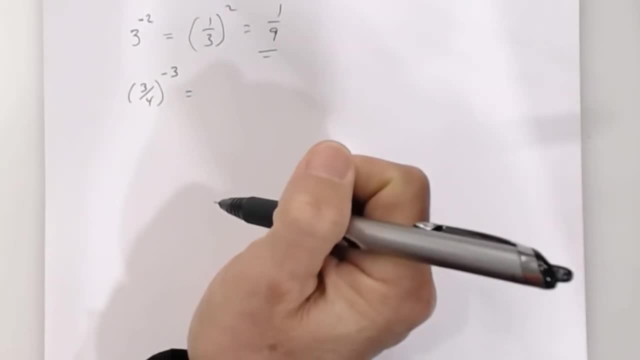 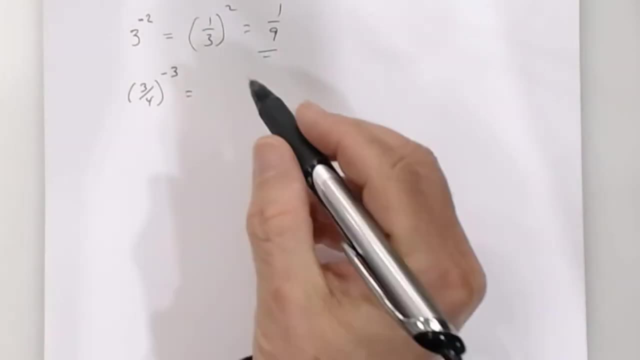 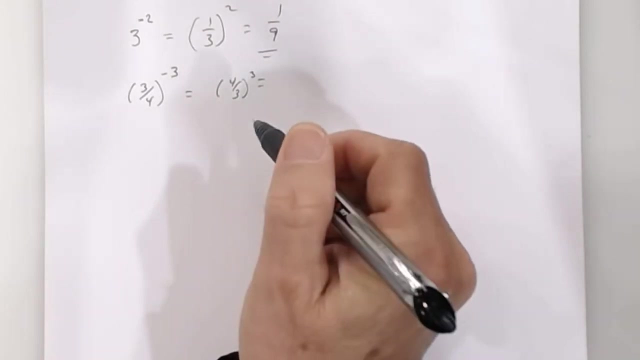 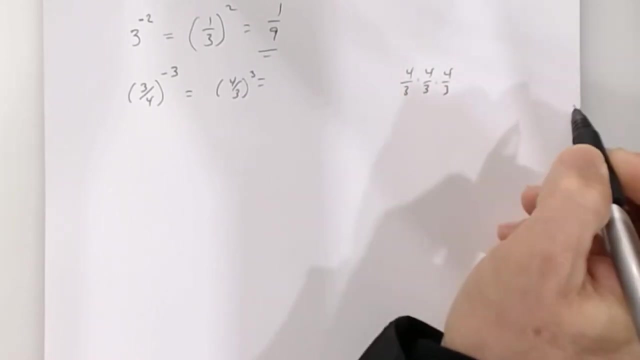 Without using the calculator. what is this equal to? How are you going to rewrite it? Four-thirds to the positive third power, And so four-thirds means four-thirds times four-thirds times four-thirds. So four-thirds to the third means four-thirds times four-thirds times four-thirds. 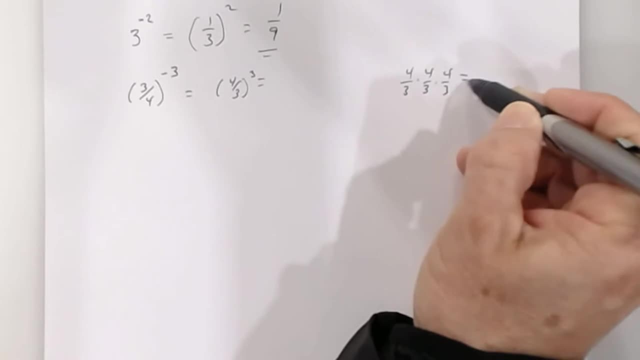 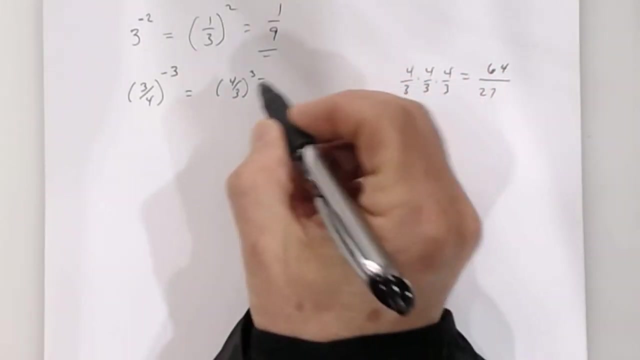 Four times four is sixteen. Sixteen times four is- And that's where you all say sixty-four. Three times three is nine. Nine times three is Okay, at least you knew that one. So what's three-fourths to the negative third power equal to: 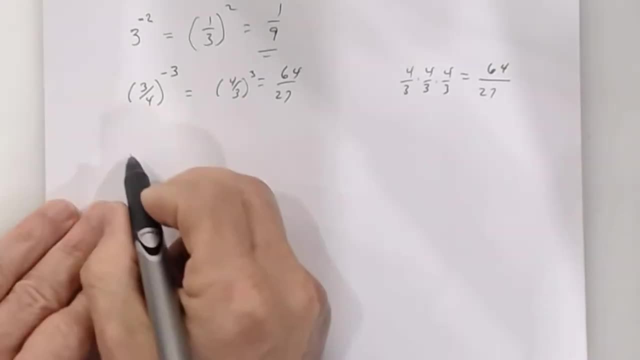 What do you say? All right now, If I have the function g of x equal two to the negative x. Now, on that in-class worksheet you had yesterday, I asked you whether that function was increasing or decreasing. And so, in this particular case, g of x, is this an increasing function or is this a decreasing function? 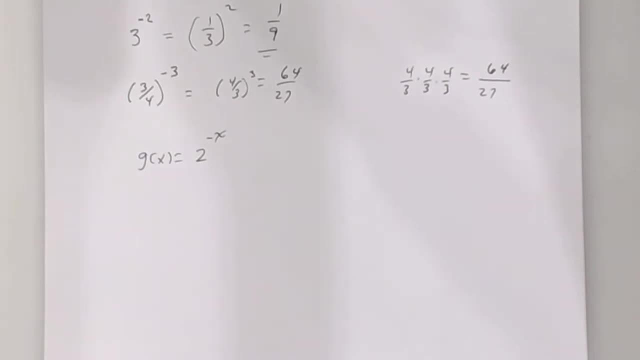 And why I don't know. there's nothing to it. I'm two Okay On your worksheet that you did yesterday in class And all of you got it correctly. so I'm not understanding why you can't tell me that one. 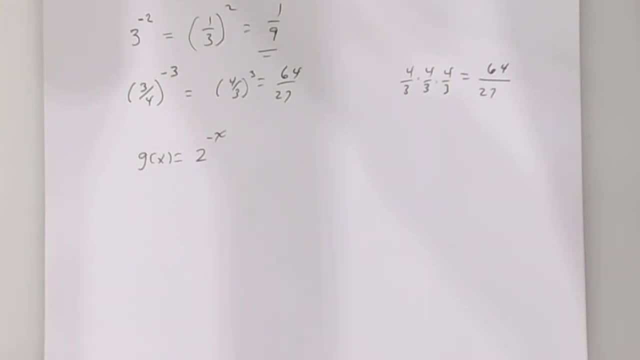 Why is it decreasing? Because yesterday we said the base is bigger than one. What's your function doing? Increasing? Well, what's the base here? What's the base here? Two, Two, Two, Three. So is it increasing? 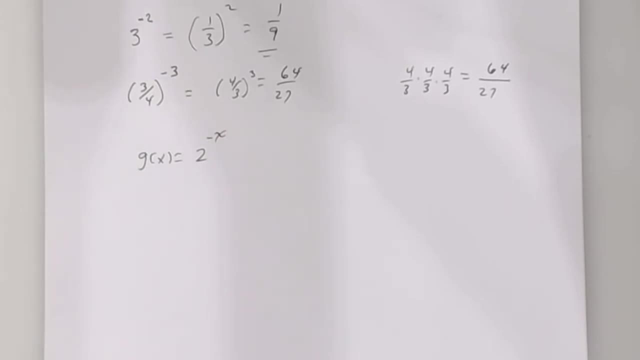 The negative exponent has something to do with it. Why do you think I talked about these two things right here. So if I'm going to make that exponent positive x, then how do I write the two? One half, One half. So this is one half to the x. 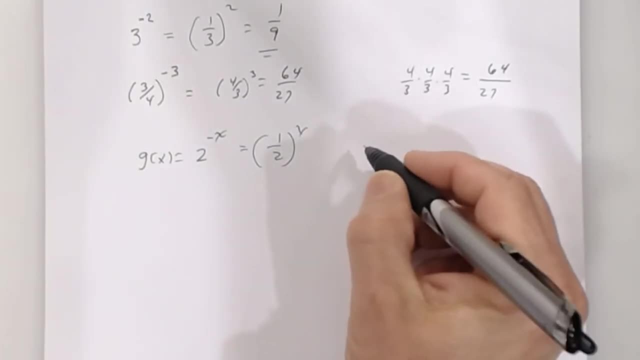 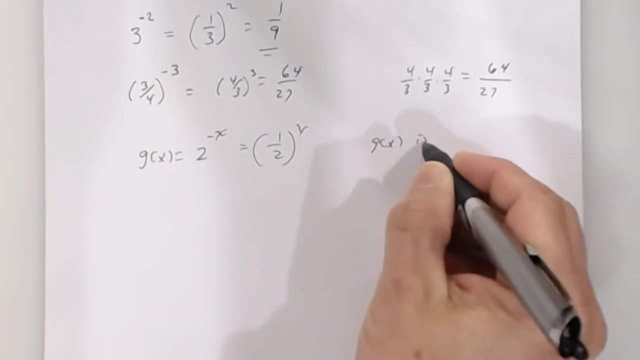 And now you're going to tell me what kind of function Decreasing- Decreasing- This number's less than one one, So g of x is a decreasing function. So there are two ways that you can graph this. Now we're going to graph. 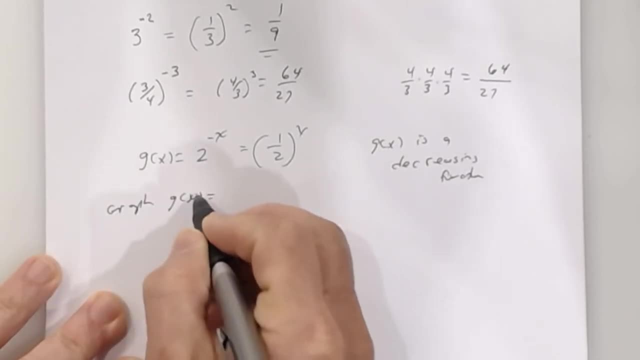 this. So let's graph g of x. So a couple ways you can do it now. You can use 2 to negative x, Or you can use what? 1 half to the x. They're both the same graph, They're both equivalent. Those are both equivalent, This negative exponent to. 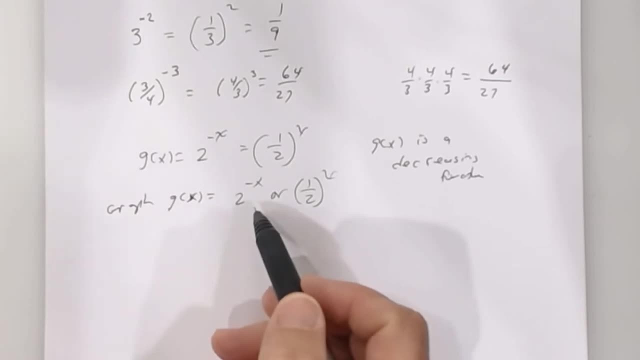 make it positive exponent. I take the reciprocal of the base. They're both equivalent, So the graph will be the same. So if you do- let's say you want to graph this one, the one that says 2 to negative x, we use the t-table, Remember. 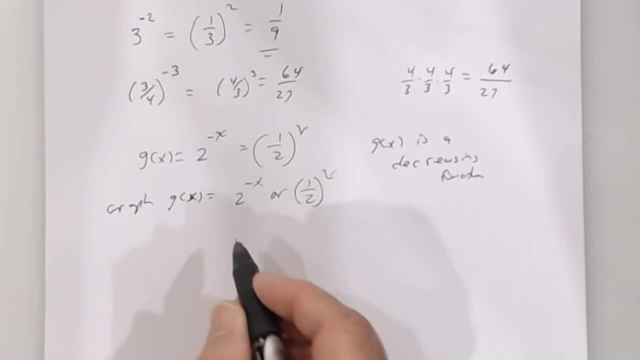 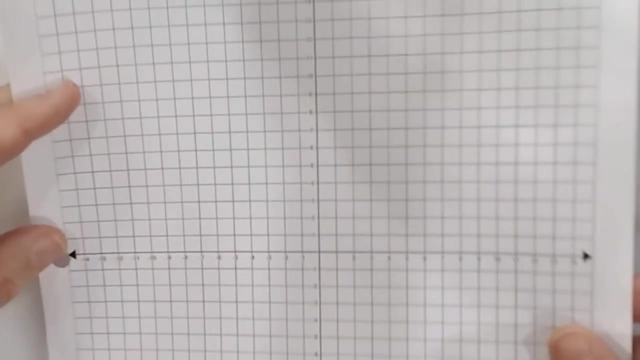 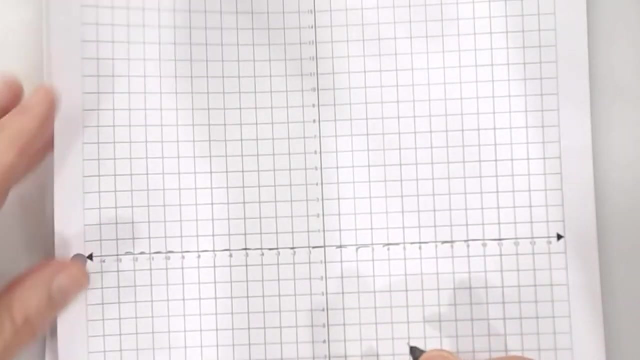 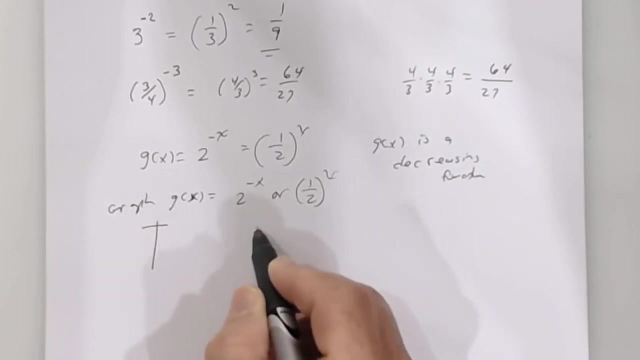 that? What's the horizontal asymptote? y equals 0.. That's the horizontal asymptote, Which happens to be which axis? The x-axis? Once we found the horizontal asymptote, what was the other thing? we had to find The y-intercept. 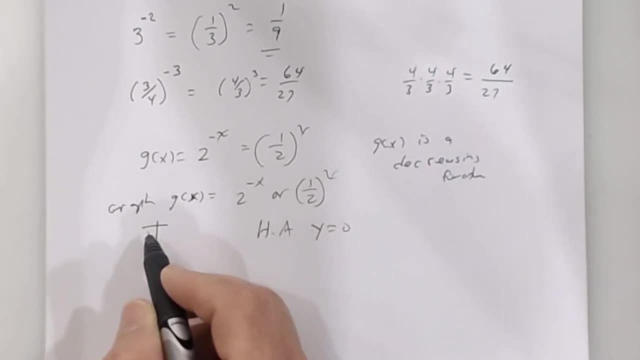 The y-intercept. And how do you find the y-intercept? Y equals 0 for x, Right? So you're always going to have a y-intercept, because what's the domain? What's the domain of an exponential? It's all real numbers, Negative infinity. 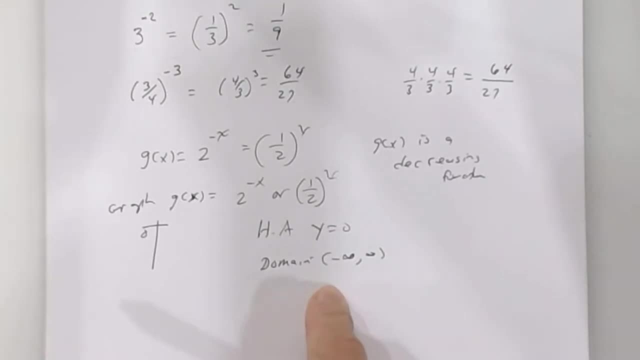 And so 0 is in here, right, Isn't? x equals 0 in here. So in a graph, when x is 0, that happens to be which intercept- The y-intercept. So you're always going to have a y-intercept. 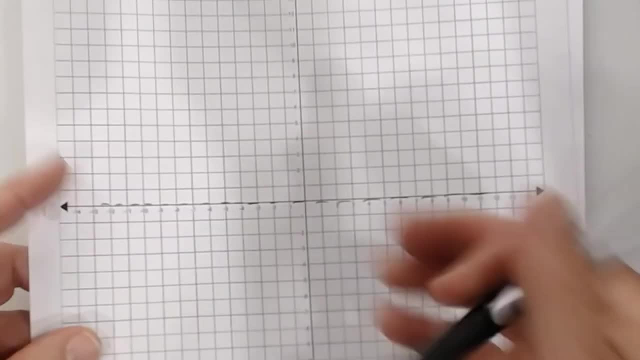 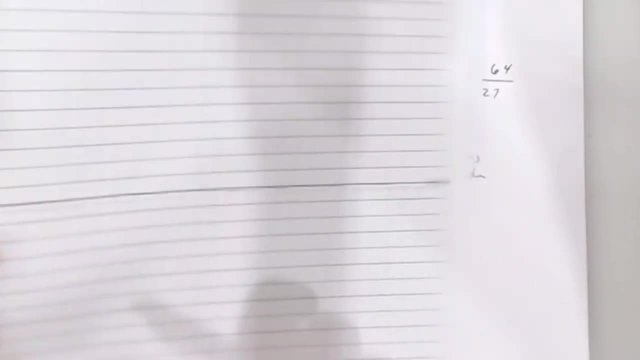 You're not always going to have an x-intercept. We saw that in many of the situations yesterday. If the graph is above or below this x-axis, it's not going to cross it. So if x is 0, I can either use this one or this one. 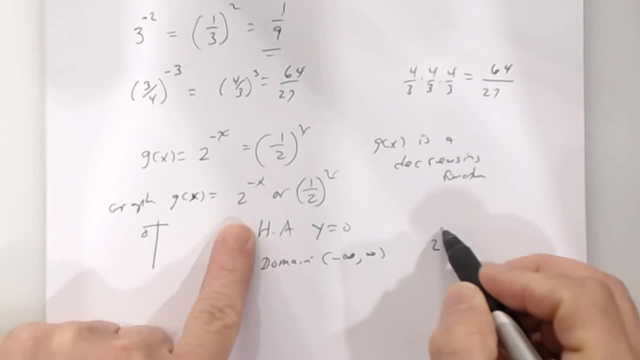 It does not matter What's 2 to the negative 0 power, It's 2 to the 0, which is what? 1.. Or if you want to use 1 half to the 0,, what's 1 half to the 0?? 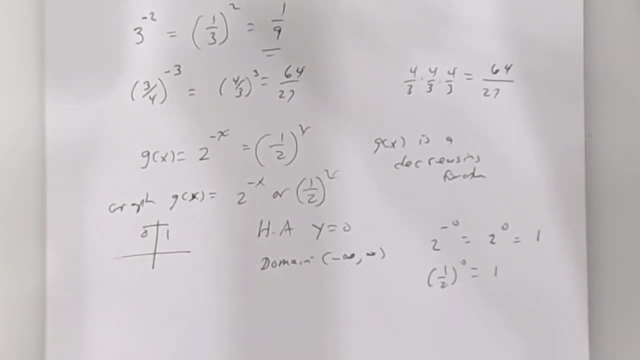 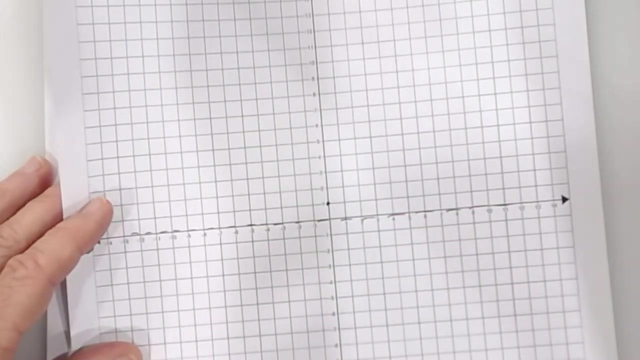 It's 1.. It's 1.. So you're, Your y-intercept is 0, 1.. So you plot that point. And now you know that the graph is located where Above or below the horizontal asymptote Above. 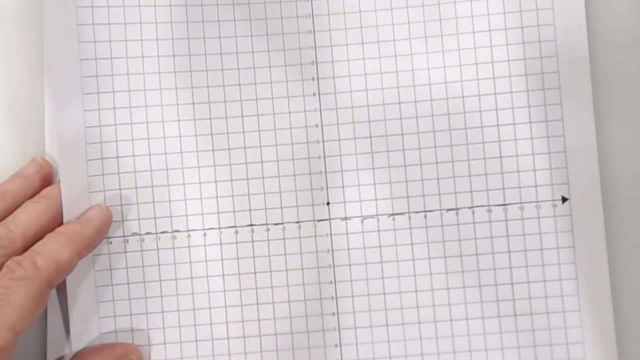 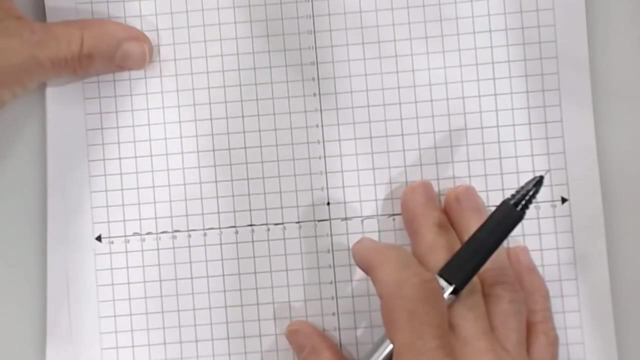 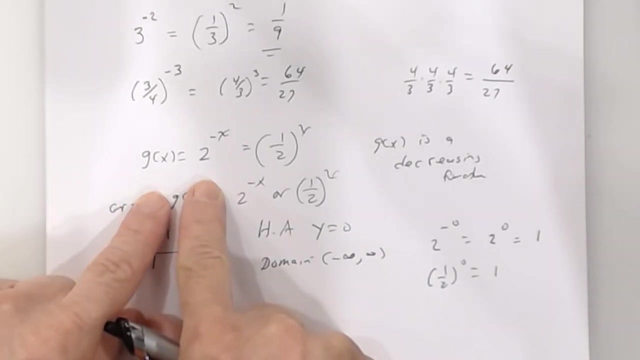 So, right away, you can tell me the range without even knowing, without even graphing it, just knowing that it's above right. And how do you know that it's above the horizontal? just by looking at your function. We talked about that a couple of times yesterday and the day before. 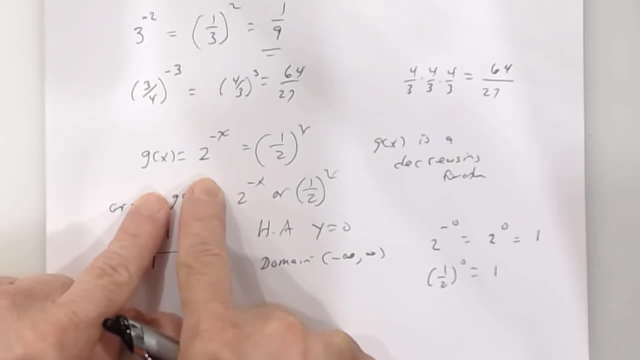 How do you know that the graph is going to be above the horizontal Guys? you know it's on your next test, right? The number in front of the base is what is What's that sign in front of? 2 to the negative x or 1 half to the x? 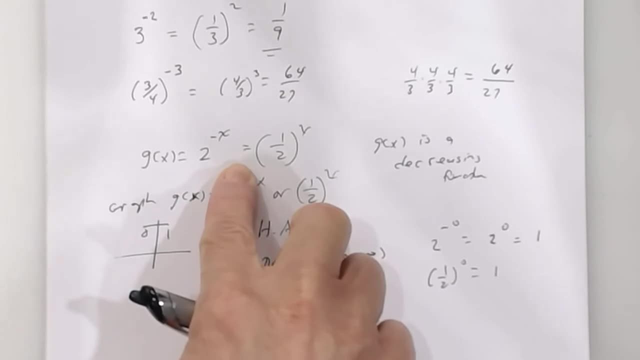 It's positive. Remember it's going to be below. if there's a reflection, There's a reflection. if there was what in front of this, 2 to the negative, x A negative. Alright, so that's on your third test, guys. 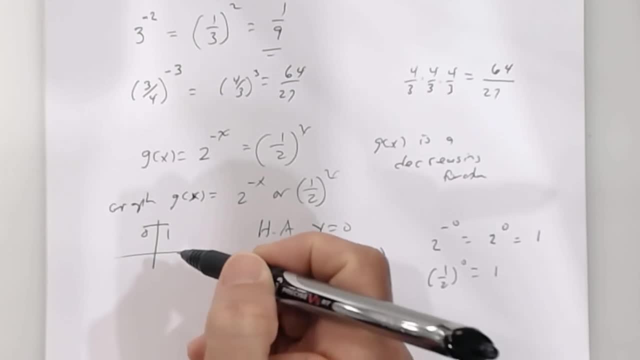 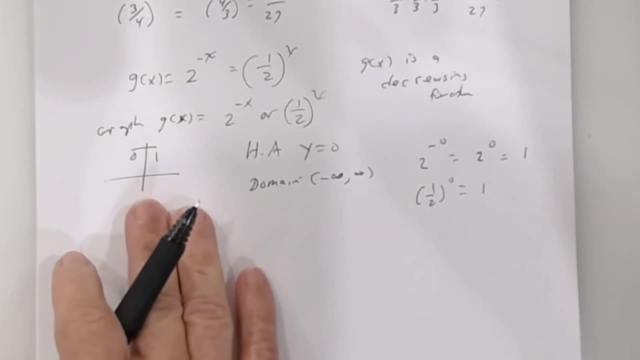 It's on your third test, Graphing these. Alright. so the graph. just without even knowing what the y-intercept is, you know that the graph is above the horizontal because there's not a reflection, And so if it's above the horizontal,